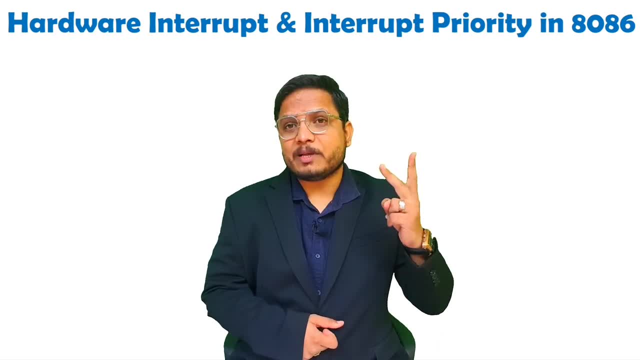 are only two hardware interrupt pins, which is there with 8086.. One is non-maskable interrupt and second is INTR. So in this video I'll explain you how exactly these two pins are used by 8086 to perform interrupt service And also I'll explain you how priorities of 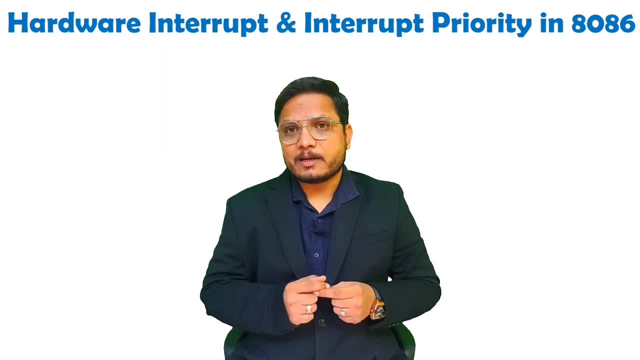 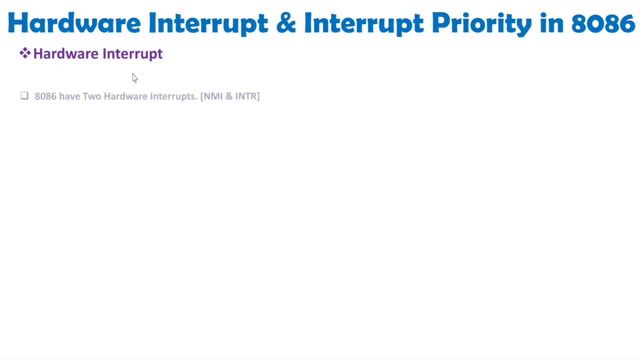 interrupt that is defined with 8086.. So let us see all those things step by step. So, my dear students, here, when we talk about hardware interrupt, then with 8086, we have two hardware pin: NMI, NMI and INTR. NMI means non-maskable interrupt and INTR means interrupt request line. So 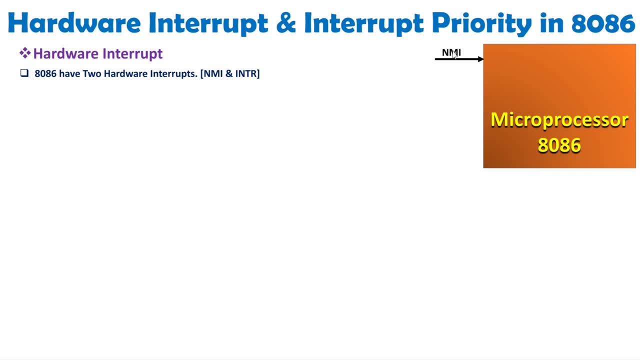 here we have 8086, in which NMI interrupt is given here and INTR interrupt that is given here. Here there are a few basic things that you should know, my dear students. NMI is non-maskable interrupt and this is vectored interrupt. Vectored interrupt means whenever. 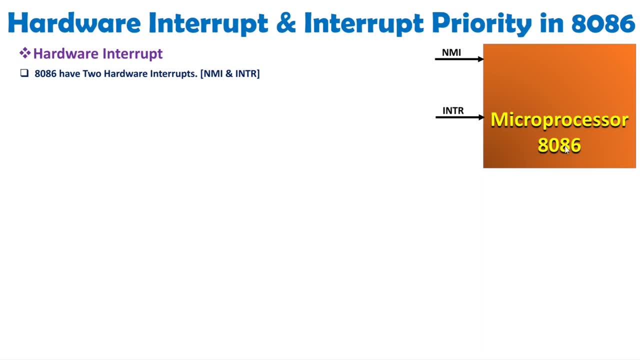 this interrupt comes here. At that time 8086 is having well-defined idea for interrupt service routine. The reason is: vector location is well-defined for this non-maskable interrupt, So ISR will get executed immediately once this interrupt is coming. But INTR, that is non-vectored interrupt. 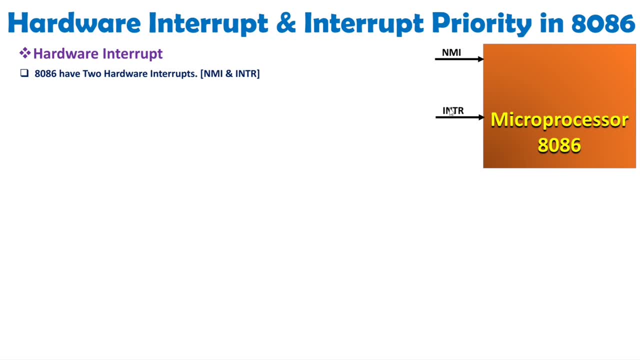 Non-vectored interrupt means what With this interrupt we don't have well-defined vector location. So with this INTR we are also using INTA bar interrupt acknowledgement. So whenever this interrupt comes, at that time 8086 will give two pulses to the device And during 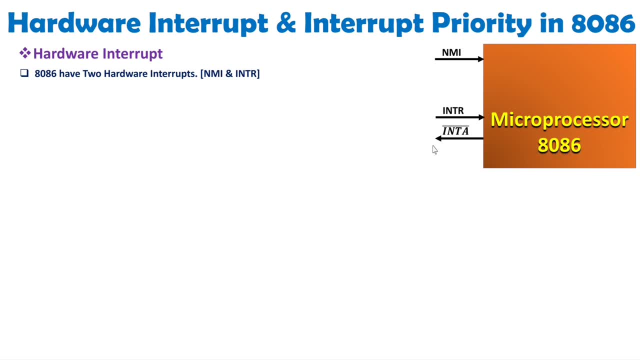 that two pulses. 8086 will take vector location for program control. So here program control should be transferred to interrupt service routine, And here with INTR It will take some time Why The reason is 8086 is not having well-defined memory location Once it receives that interrupt. 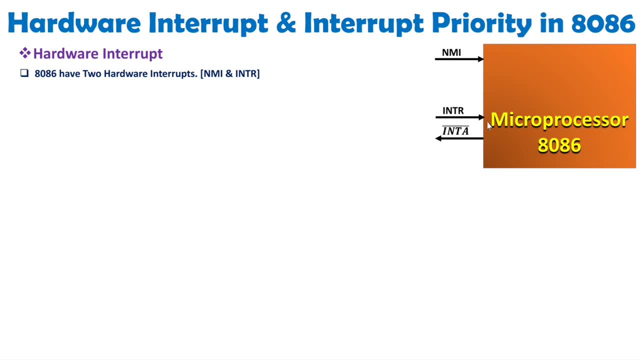 it will be giving acknowledgement, Then it will take address of that program control and then it will give service. So this INTR interrupt is slower than NMI. But, my dear students, this is slower doesn't mean that this is not essential. There are. 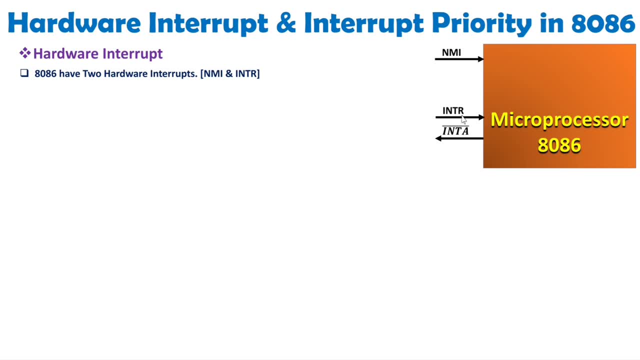 things that we can do by using INTR. I'll explain you how to have multiple interrupt acknowledgement even So, here let us see first basics of NMI and INTR. So, my dear students, NMI is non-maskable interrupt. It is having highest priority in hardware category. that. 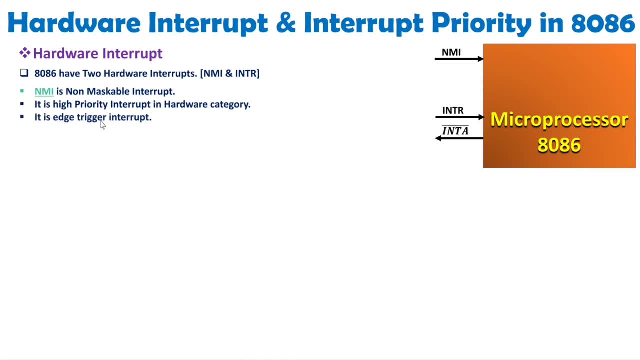 you can say, and here it is, age trigger interrupt and when it executed in 8086 at a time there will be type 2 interrupt. that will happen and in type 2 interrupt how execution is happening. for that I have made separate video that is IVT interrupt vector table. in that we have 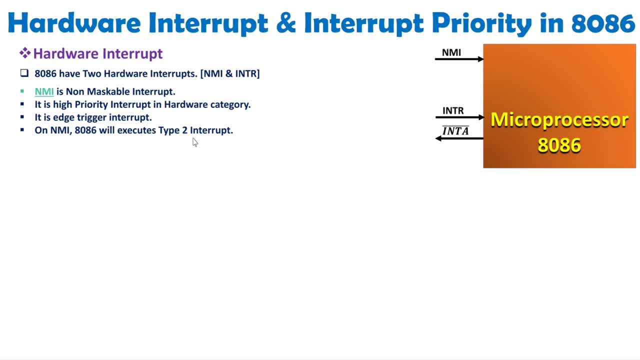 seen that in detail right Now. my dear students, you should know when NMI is getting executed. ISR address: that is there at this memory location, 000008 hex. that is there as per type 2.. You see 2 into 4, that will be 8 hex address, right. and my dear students, with this type 2, with 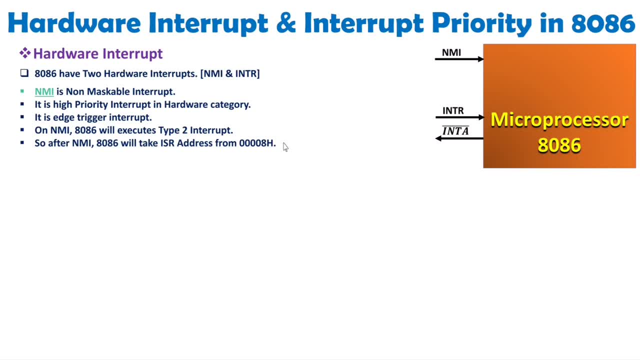 this address we are having total 4 bytes and those 4 bytes are having value of CSNIP that we need to load it for ISR address right. So NMI, that is, having well defined address allocation for program execution right, but that is not the case which is there with INTR. So, my dear students, INTR is interrupt request. 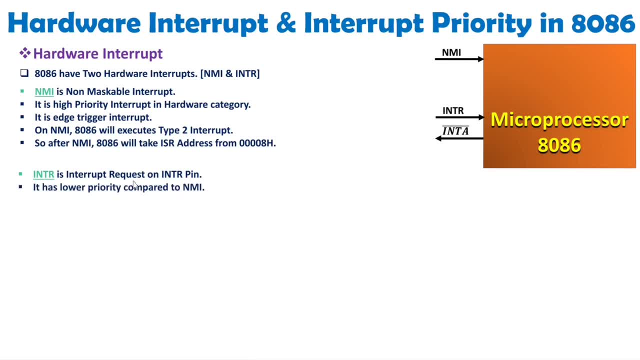 line in that you will have to see how we need to take address of that program control. for that INTA bar is used and it is having lower priority compared to NMI. that you should know right Here. it is maskable as if interrupt flag inside 8086 that is 0, then it is not. 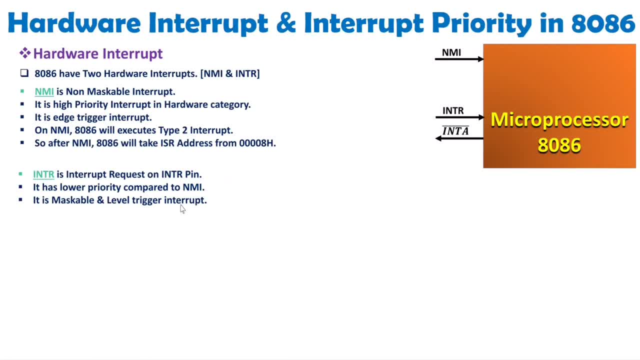 the case. So you should know that when this interrupt can not get recognized, that you should know, and this is level trigger interrupt, This NMI, that is age trigger interrupt, and this INTR, that is level trigger interrupt Here, my dear students, when INTR that is been, 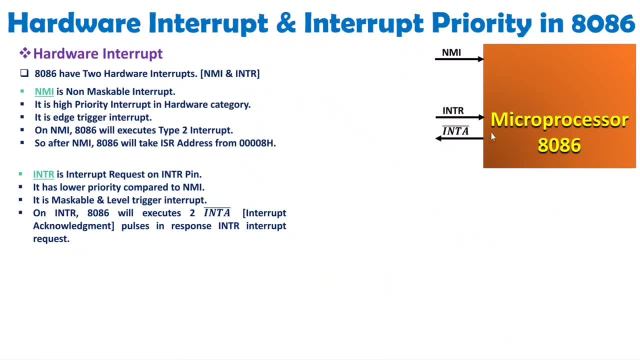 received by 8086. in response to that, 8086 will give two pulses on INTA bar right and those two pulses are used to get IDR equal to 0.. This is the level trigger interrupt, This NMI, that is age trigger interrupt, and this INTR, that is level trigger interrupt. 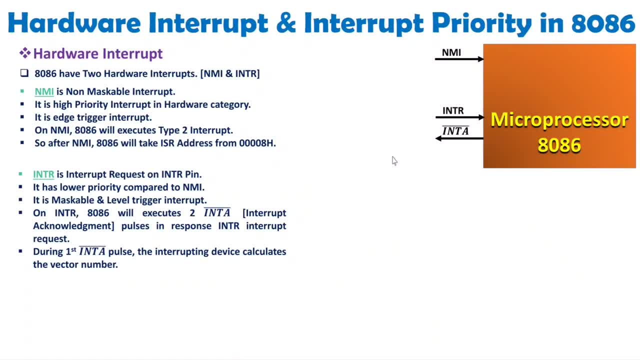 used to take address at which ISR will get executed. So during first INTA bar pulse interrupting device will calculate vector address number and in second INTA bar pulse interrupting device will sends vector number of INT instruction right. So after having execution of this second INTA bar pulse, 8086 will receive that interrupt number and based on that service, 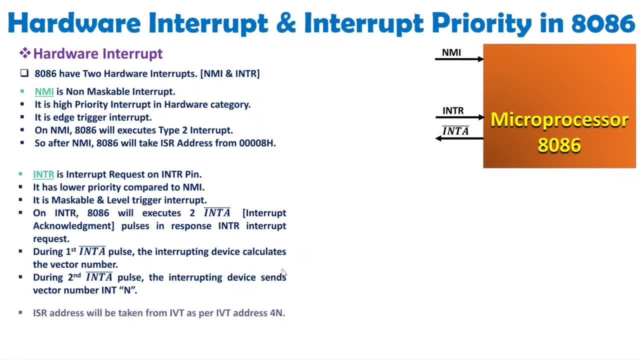 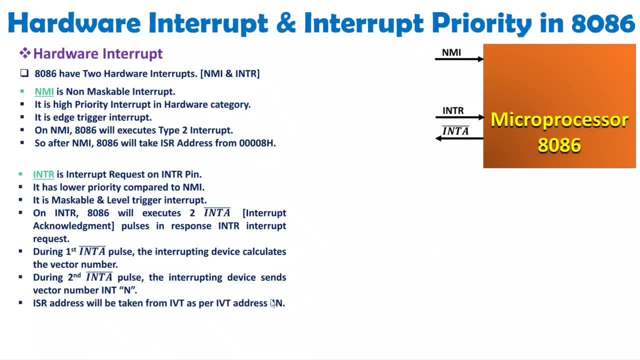 That will be the address right and at that address, whatever CSN IP that is there, that will be loaded for physical address and then ISR will get executed right. My dear students, here, IF is equals to 0 will not allow INTR interrupt service right. So you should know. 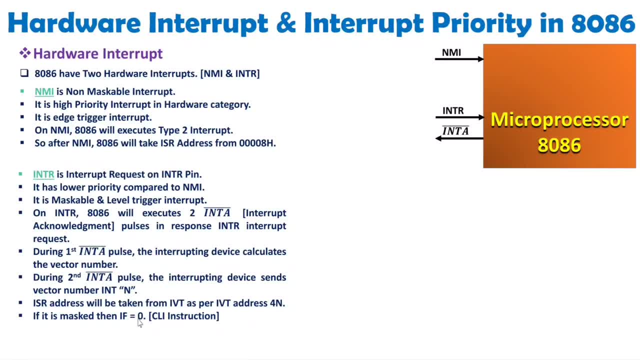 to mask INTR IF is equals to 0, that we need to have and that we can have it by C L I instruction. clear interrupt flag instruction. right, And if you want to unmask, in that case you should make it to 1 and that we can have it by having set interrupt flag instruction. 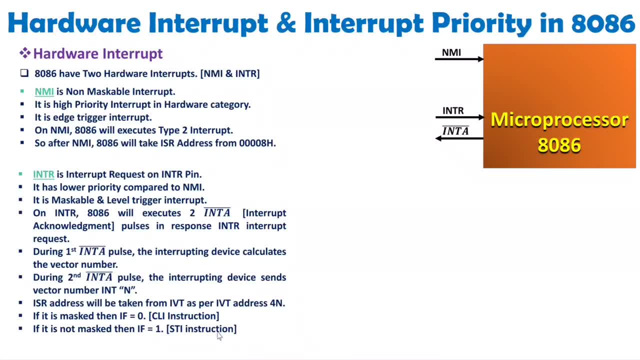 H, T I instruction right. So these are the basics of NMI and INTR. Now, as I have told you, my dear students, with 8086 we just have two hardware pin, but by this time we will have this INTR. we can have many hardware interrupt service. How you see, as if you. 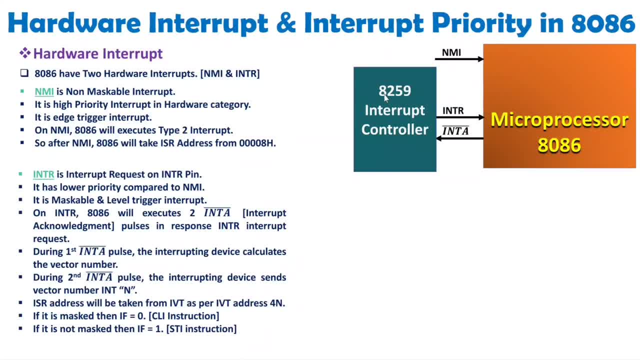 use interrupt controller, then 8259 interrupt controller can handle 8 interrupts and this 8259 will identify priorities as well. right, So here what we can do is here we can program this 8259 for 8 different interrupts and, as if you wanted to have 60 interrupts, we can. 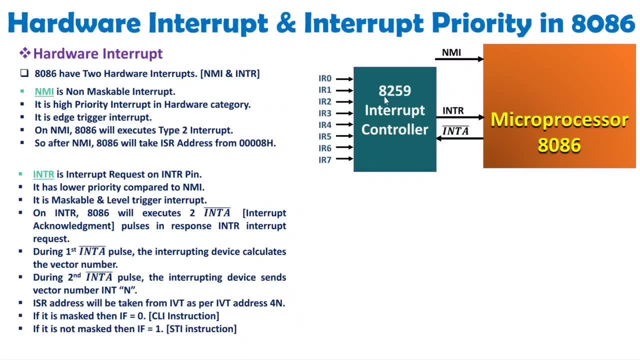 have 60 interrupts. then here, my dear students, one master 8259 can be interfaced with another slave 88259, and then we can have total 64 interrupts. So 64 interrupts can have service via this two lines only, right. So 8086 is having only two hardware interrupt pin. But 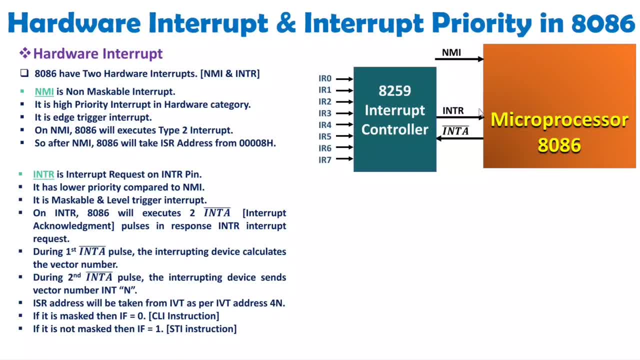 this INTR pin that we can use it for many interrupt controls. That's why this is very essential. It is having lower priority, It is slow, It is fine, But by having these two terminals we can interface as many interrupts as you wanted to. 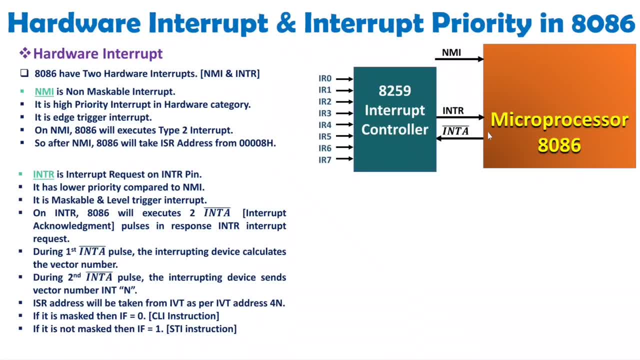 have Right. So that's why these two terminals are very essential. Now, my dear students, let us see how priorities are there with 8086 for interrupt. So when we talk about highest priority, that is there with software interrupt. you should know INTN, Those are software. 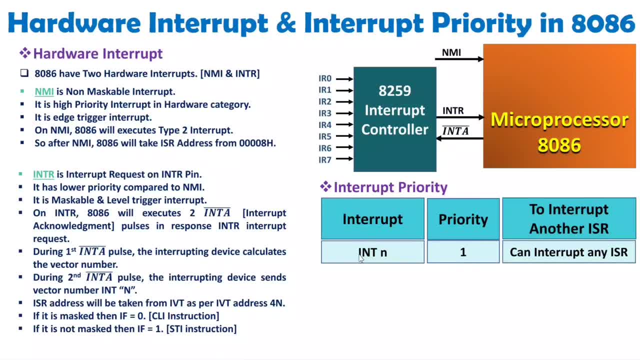 interrupts which we have Right, Total 256 software interrupts are there. that is having highest priority, and the software interrupts can interrupt any ISR that you should know. So for example, if you are giving service to one interrupt in between, that if this: 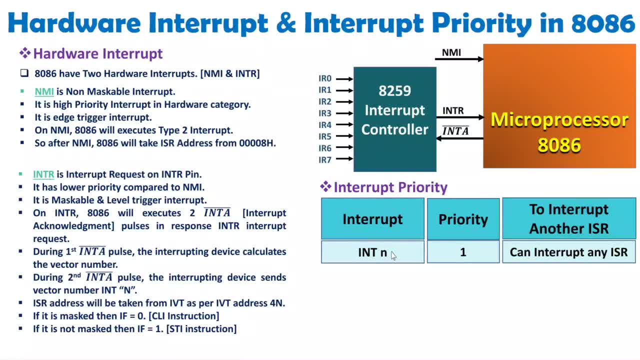 interrupt is arising, then you will have to execute that interrupt as well, Right, So it can get executed during isr as well. here, my dear students, second priority is there with non-maskable interrupt. this is there in hardware category, right, and it also can get executed during any isr. 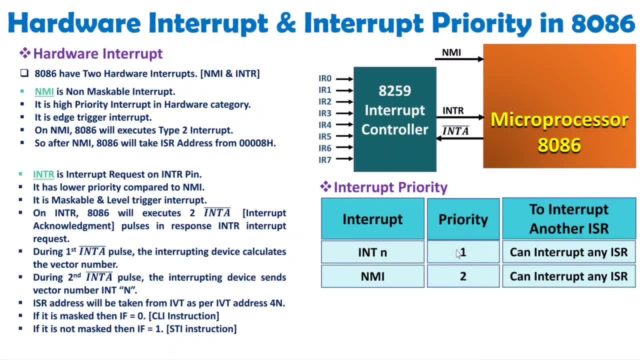 priority means what, my dear students? if simultaneously two interrupts are happening, then you can say which one should get executed right. and in program you cannot execute multiple int instruction. that's why you can say: it is having highest priority, all are having equal priority. that even you can say: but nmi, that is hardware interrupt right, that can execute that.